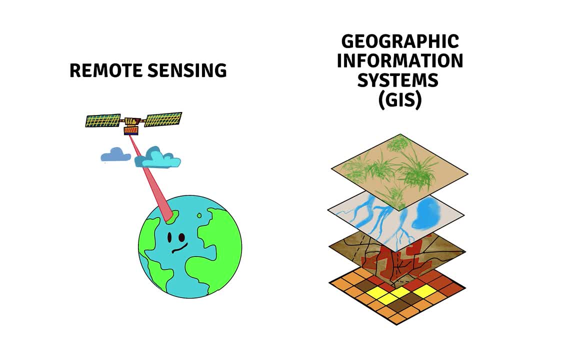 examples of applications of remote sensing and GIS and will be discussing the kinds of remote sensing technologies we currently have. We will also be touchpasing some of the key terms associated with GIS towards the end. I have separated the video into chapters so that, in case 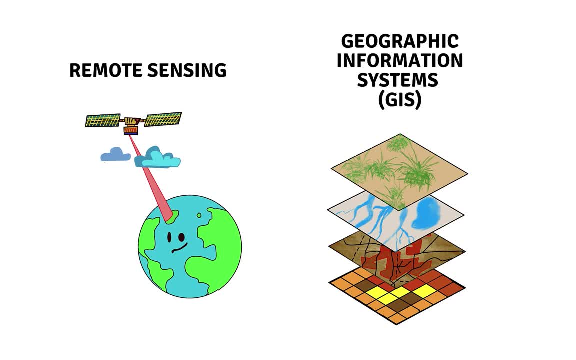 you are interested in a specific topic, you can hop onto those sections, and all the links mentioned in this video will be included in the description section below, So that, out of the way, let's get started. Hey guys, welcome, or welcome back to my channel and happy new year, If you guys are new. 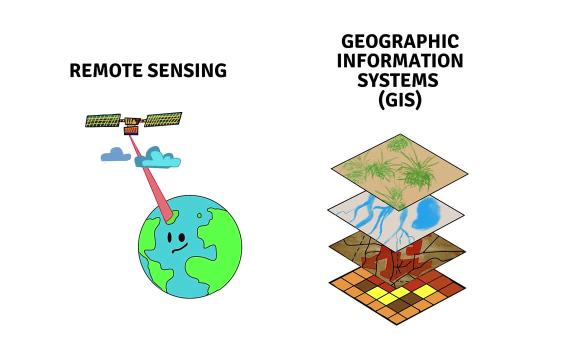 here. hi there, this is Mikey. I'm a PhD student at UC Berkeley, working at the intersections of remote sensing for a student. I'm a PhD student at UC Berkeley. I'm a PhD student at UC Berkeley and I'm a PhD student at UC Berkeley. I'm a PhD student at UC Berkeley. I'm a PhD student at UC Berkeley. 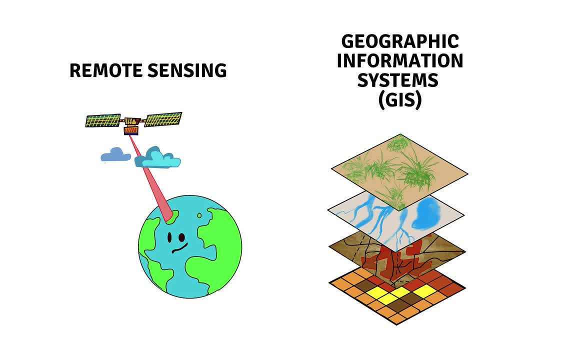 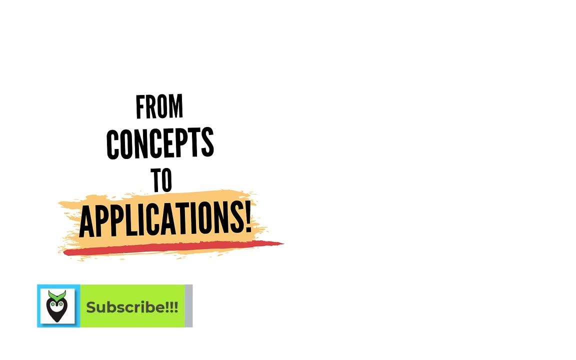 And in this channel I'll be posting daily videos on topics ranging from drones, ladder trees, maps, data analysis, visualization, machine learning and everything else in between. The idea is to make concepts associated with physical geography and data sense simple enough so that 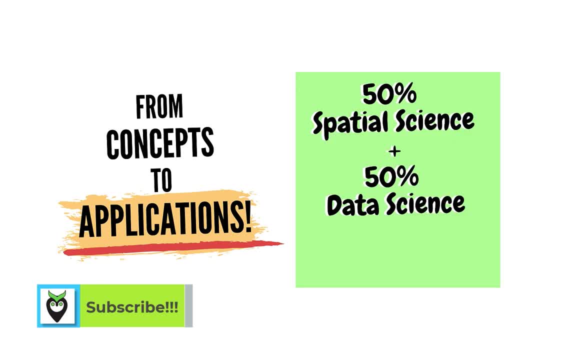 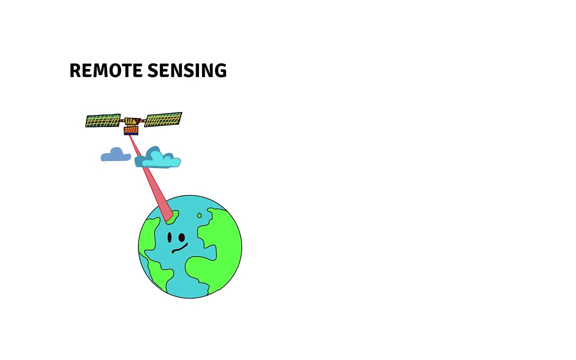 more people can apply it. So, yeah, this channel is going to be a bridge between spatial sense and data sense, So if you're into any of this, make sure to subscribe. Okay, let's start with remote sensing. When we first hear remote sensing, what are those things that we associate it with? Well, 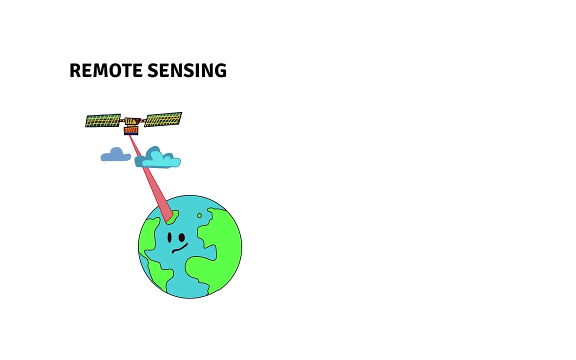 satellites and obviously NASA, right. That's why here I got this makeshift drawing representing a satellite drawing and also the confused earth. But remote sensing is much, much more than just satellites, which we'll be getting into in a bit. So what is remote sensing? For answering that, 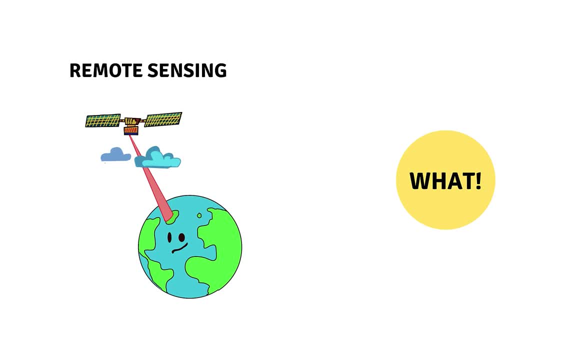 let's split the words here. The first part is remote, This relates to something that is not physically touching the object of our interest, And the second part, sensing, can be interpreted as a feeling we get when we sense an object. So by feeling in this case we mean the information that we are extracting, which can be 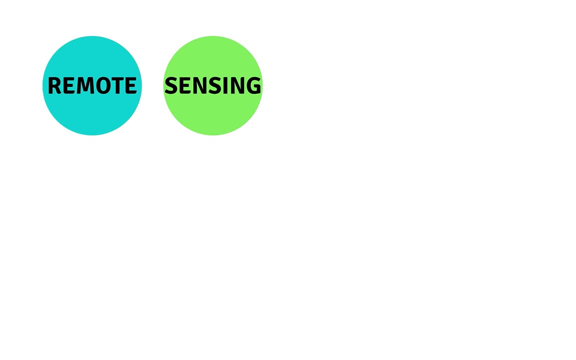 something like a physical property of the object. And this is exactly what remote sensing stands for. It is a sense of measuring or obtaining information of an object without making any physical contact. I repeat: remote sensing is a sense of measuring or obtaining information of an object without making 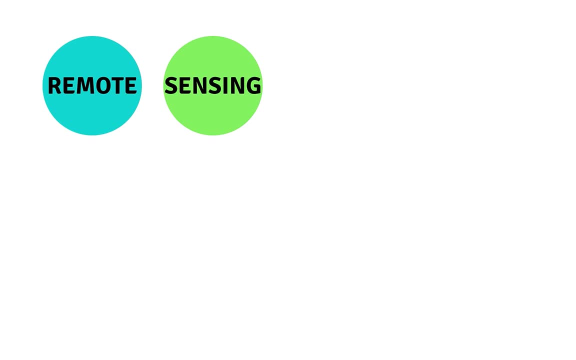 any physical contact, So without making any physical contact. that's the important part here, And the term was coined in early 1950s And nowadays it's a major branch of study within the realm of physical geography. Let's consider our day-to-day behavior and see whether we can relate it to the concept we just discussed. 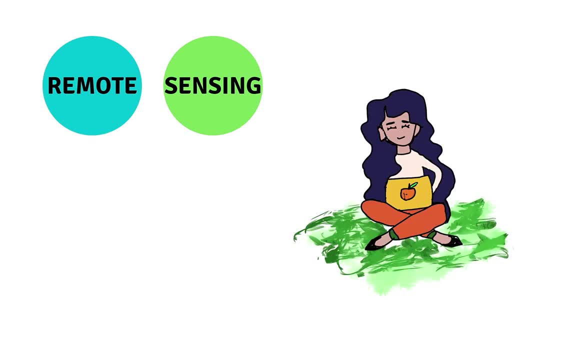 For instance, imagine you're hanging out at your backyard and working on some assignment in your laptop. So are you here remotely sensing any data? If you consider you're typing on the keyboard, it is not remotely sensing the data as you're making physical contact here. This is the same when we take the case of lab work. 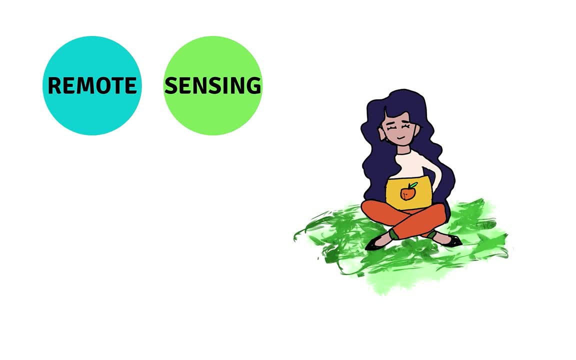 where we are performing experiments and physically measuring things, Whereas, imagine, here you got bored and you decide to relax and just look around and observe the trees and birds around the corner. This can be considered as remote sensing, as here you're not making any physical contact with the object of interest. 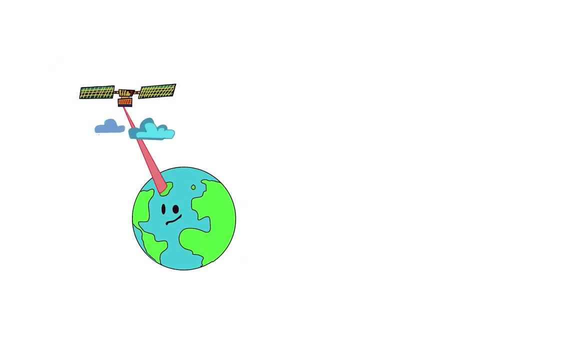 As I mentioned before, even though satellite-based imagery is the most popular topic related to remote sensing, remote sensing doesn't have to be all the time All is done from outer space Nowadays. drones are another widely used platform for performing remote sensing. 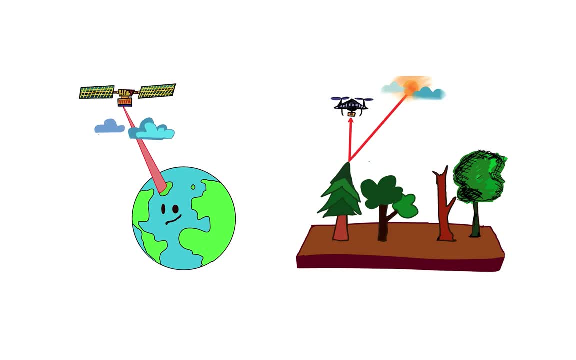 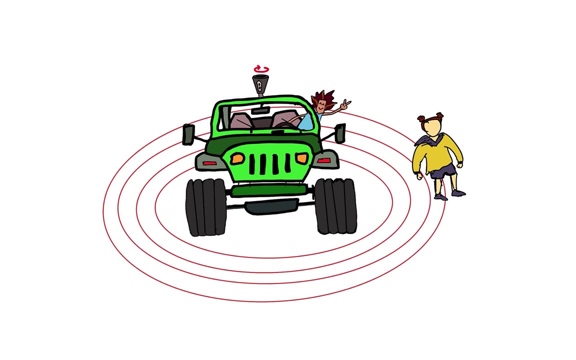 Also note that the platform carrying the sensor don't always have to be in the air. The laser scanning technology now that's being used in the autonomous car is also an example of remote sensing. So is the x-rays you take at the hospital In case of the laser scanning technology, which is also known as LIDAR. 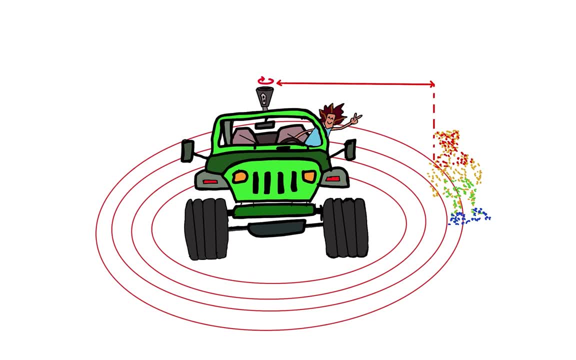 we are able to detect objects and even create three-dimensional models of them. I'll be creating a playlist entirely on LIDAR remote sensing in the coming days and the link will be included in the description section in case you are interested in exploring more on the topic. 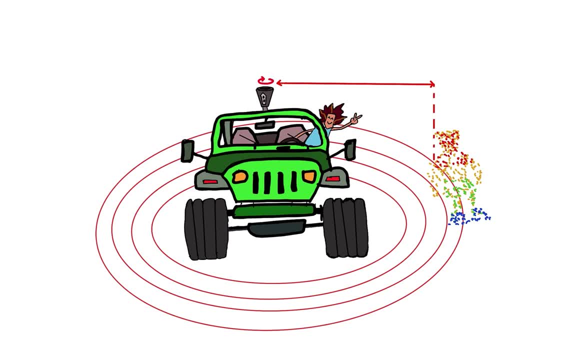 Among all the examples we have just mentioned, note that there is always a sensor that collects the data and there will be a platform for having the sensor, whether it be a satellite or drone or car, And based on how the object under focus is illuminated. 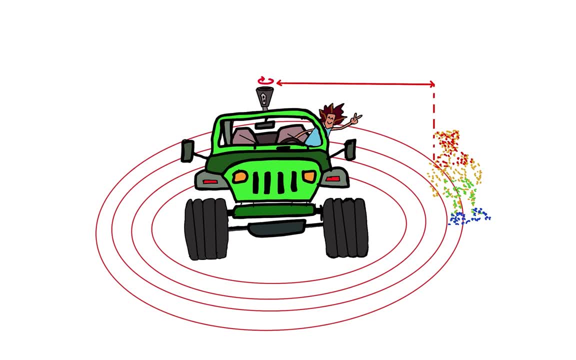 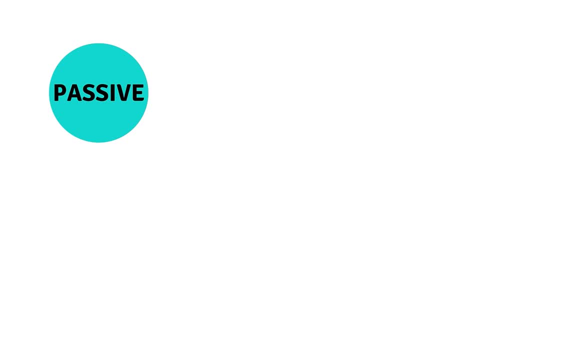 remote sensing can be classified into two categories: active and passive remote sensing. In case of passive sensors, such as drones taking photos, here it depends on external energy for illumination. They actually measure the reflected sunlight emitted from the sun. Meanwhile, active sensors, they have their own source of energy for illumination. 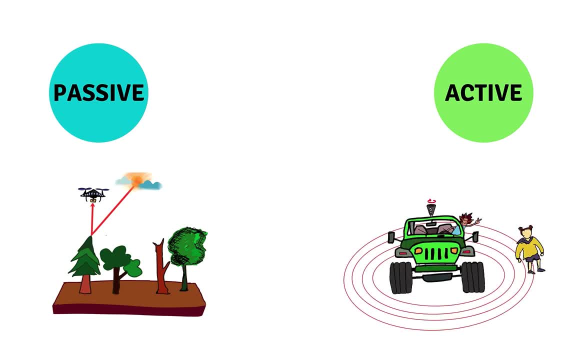 and LIDAR is a classic example of this. Another relatable example can be when you take a photo on your phone at night using flash. Here you use your own source of light for illuminating the television, So this is also an example. 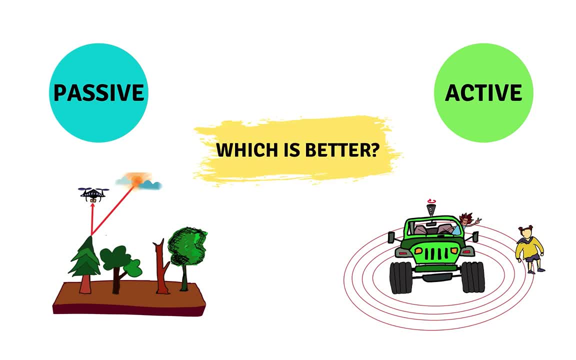 Now, if you ask me whether active remote sensing or passive remote sensing is better, it totally depends on your particular situation. In general, active remote sensing can be found to be more dependable than passive remote sensing methodologies. As you can imagine, we can't depend on satellite imagery based on remote sensing during the night time. 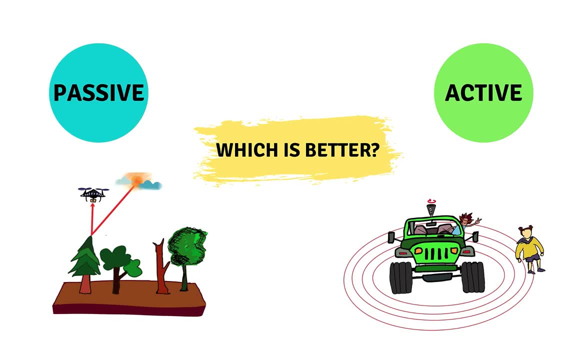 as we need the sun's energy for illumination. Also, these sensors are heavily affected by things like clouds and aerosols. However, active remote sensors are more effective. They are mostly more expensive than passive remote sensing technologies, and it's not always possible to acquire such data for large scale or recurring studies. 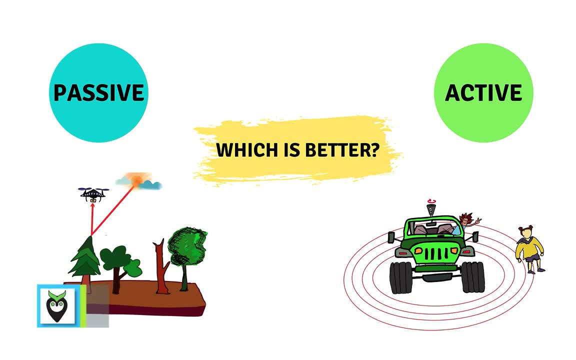 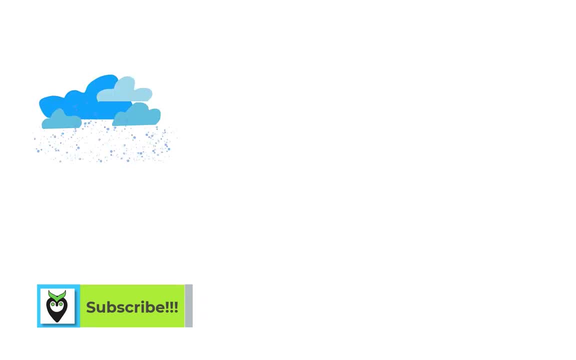 I think this is a very broad topic and deserves a video of its own. Let me know in the comment section if you guys would like me to make an in-depth video on this in the future. Well, we live in a world overloaded with data and, apart from the personal level data collection happening, 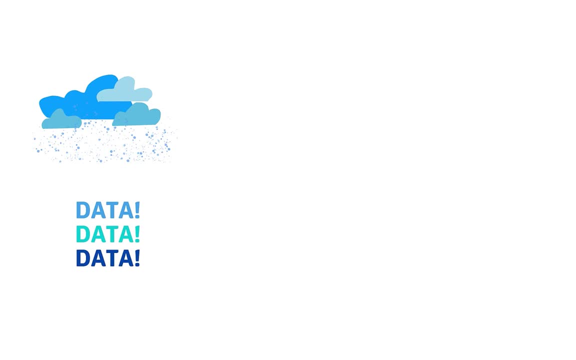 there are also a lot of other global scale active and passive sensors that are orbiting the globe and collecting data of the earth 24x7.. Even though we won't be going in a lot of detail here, I would like to introduce you to some other major types of remote sensing. 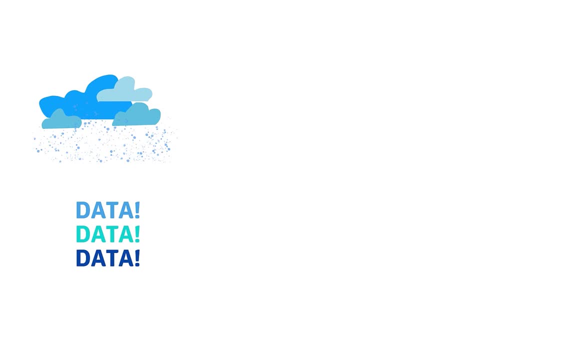 All these classifications are primarily based on the electromagnetic spectrum. you know the thing we all learned as we were kids? Yeah, the same thing where the visible light falls towards the center. Without doubt, the most common and widely available remotely sensed data is through optical remote sensing technologies. 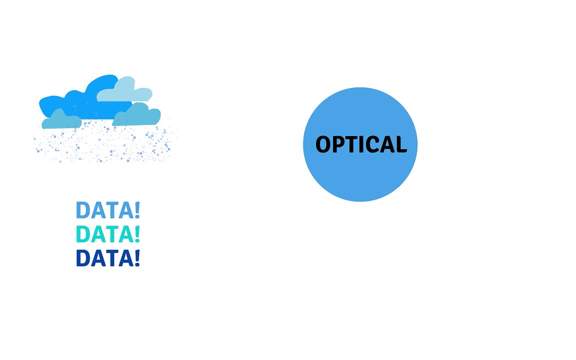 Optical remote sensing makes use of visible near-infrared and shortwave infrared sensors for capturing images. Another common remote sensing method is the LIDAR, which stands for light detection and ranging, and this is an active sensor where the target is illuminated with laser light and the reflection is measured with a sensor. 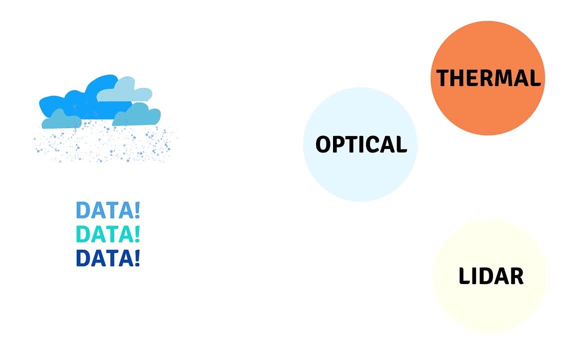 Then we have thermal remote sensing, which uses the infrared portion of the spectrum and measures emitted thermal energy, And another remote sensing technology that is gaining popularity is the microwave remote sensing, which uses the infrared portion of the spectrum and measures emitted thermal energy And, once again, based on the source of energy. 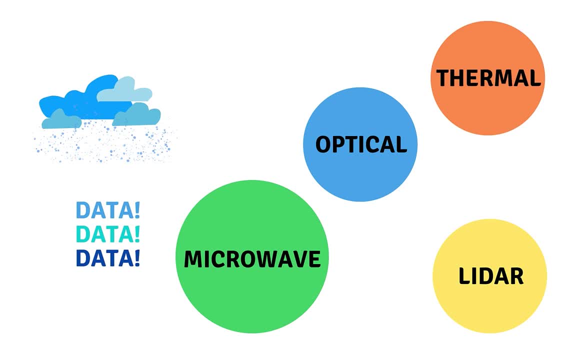 all these remote sensing technologies can be further grouped into either active or passive sensors. Now, after realizing that we have all these data, so what's next? A lot of us are oftentimes left with a bunch of question marks inside our head, and it's totally normal. 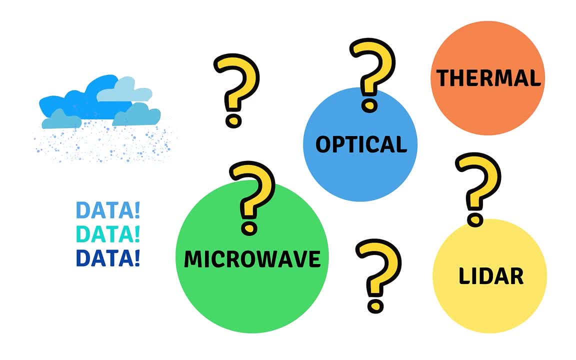 Based on our interests and research questions, we need to decide what kind of remote sensing data to choose from. For instance, a person working on the agricultural sector might find microwave remote sensing very useful, as it helps quantify properties such as soil moisture, Same with optical remote sensing technologies, which will allow you to monitor plant health and estimate crop yield. 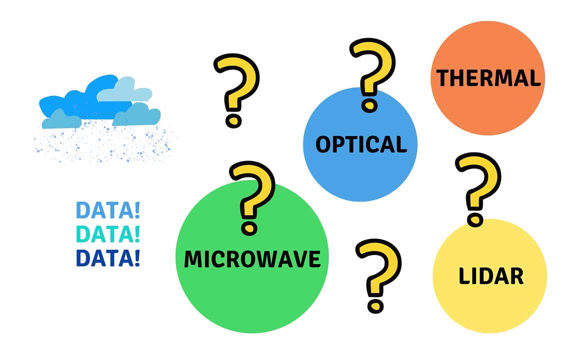 On the other hand, a person working in the urban designing might be more fascinated with LIDAR, as this can be used to develop something like 3D models of the buildings or bridges. Respectively of the field you are in, I bet you can find some applications of remote sensing in your everyday work. 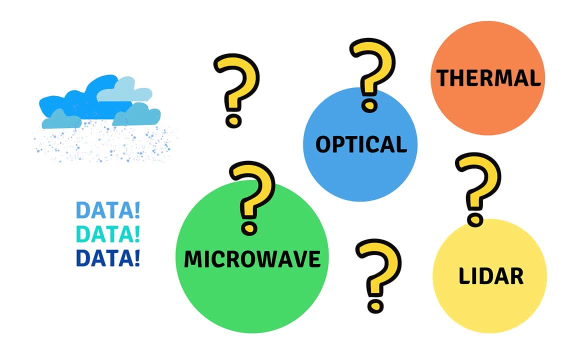 We just scratched the surface here. There is even more. We also have something called sonar, which utilizes sound energy and make observations based on how sound waves bounce off various objects. Same way, we also have radar, which we all know is something used by police for speed enforcement. 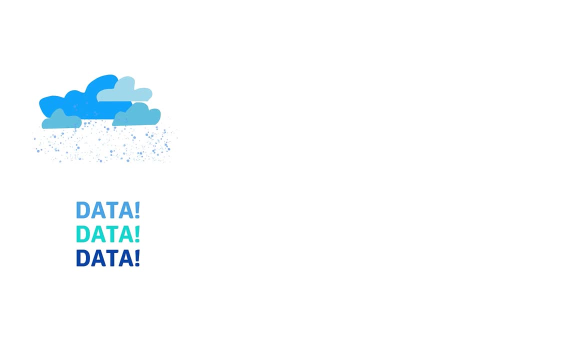 But once again, make sure not to get overwhelmed with all this vast multitude of data. I know this might be a bit too much for an intro video, but I just wanted to give you an idea of what all you can do using remote sensing. 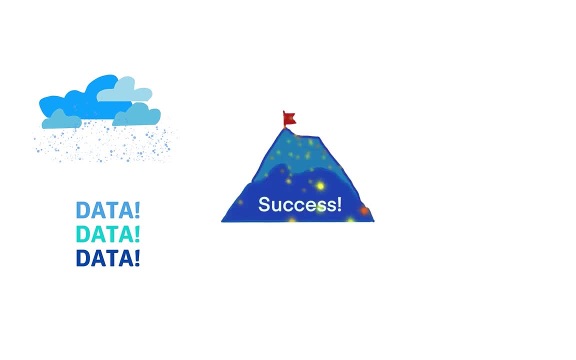 Nowadays, we just see the success stories of people coming up with all these amazing discoveries using the data available, But we should also remember that all these are achievable for us as well. The thing that is holding a lot of people back is not the lack of information. 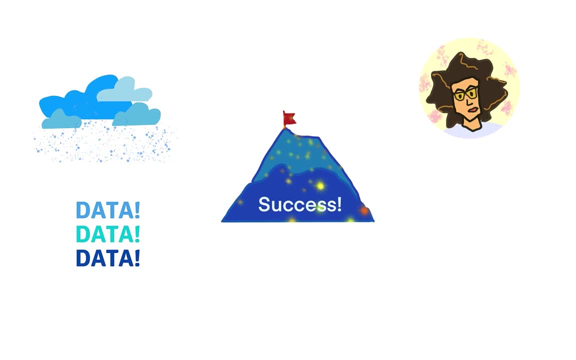 but the surplus of information. Imagine you see something like this: A satellite used to detect forest fires in Amazon or something like that. And now, if you want to try doing the same, you are generally forced to read an entire textbook or numerous research articles. 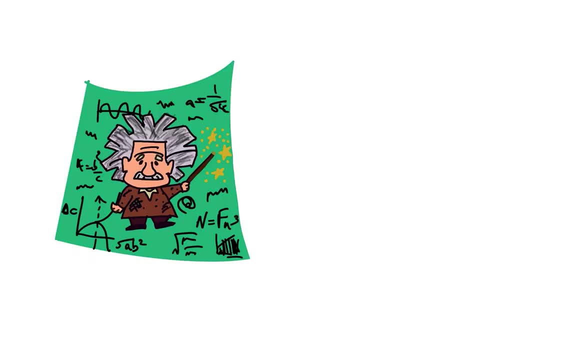 All these long-winded research explanations are for sure required, But you also need to make sure that the tools are easily accessible to the common public and are easily understandable so that more people can get involved, And that's a major motto. That's a major motto of this channel. 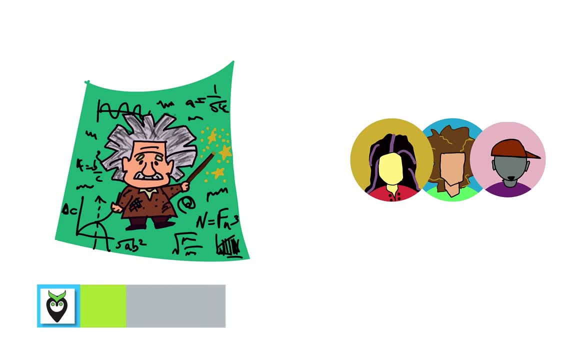 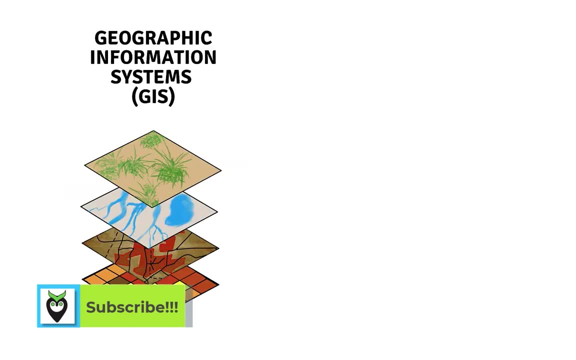 So if you agree with my ideology, hit that like button and make sure to subscribe. Okay, so now let's move to the second part of this video, which is GIS. GIS stands for Geographic Information Systems. At some places, I have even seen it expanded as Geographic Information Science. 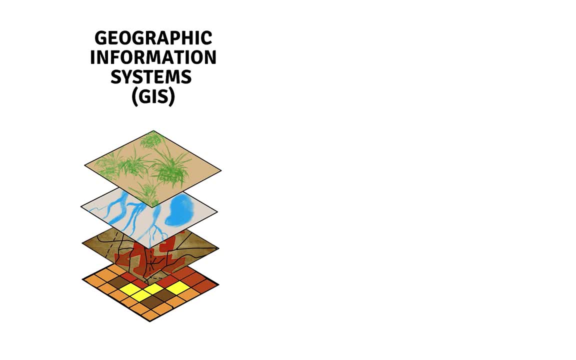 I drew this figure as layers of something that you easily associate GIS with. However, the most important keyword regarding GIS is the location. This helps us understand what has happened at a particular location, what is happening now and what can happen in the future. 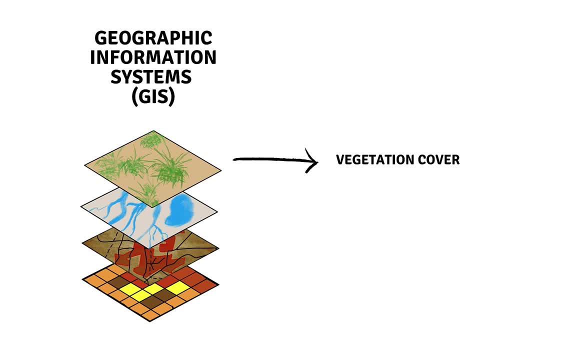 Let's say, the layers here represent the vegetation cover, water bodies, streets and political boundaries. This is an example of how we can split an area using GIS. We separate a region into multiple layers so that it's easy to analyze the situation and make decisions. 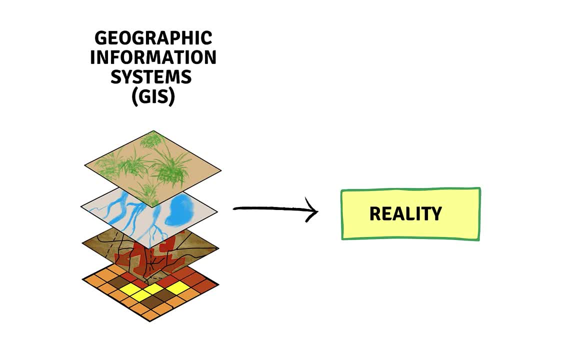 For example, if you want to buy a new home in a given locality, using GIS layers you can evaluate how much time it will take to reach the airport from this housing location. Are there any rivers nearby? Are there any hiking trails in your area? 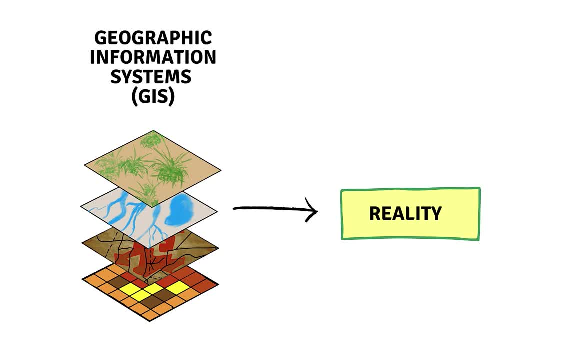 Or even something like the population density or area of your respective county. You might not be recognizing it, but you actually make use of all these concepts on a daily basis, while using apps such as Google Maps. So back to the real deal. what is GIS? 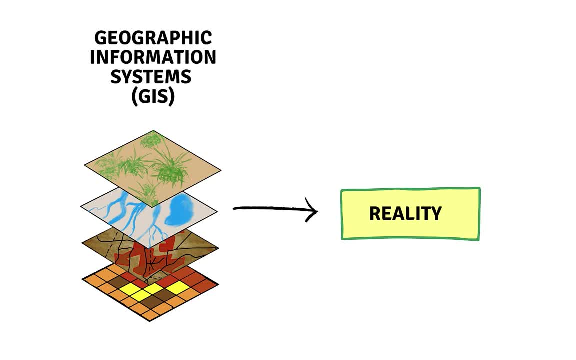 This is a very hard question to answer, you know, as there are a hundred ways to answer this. However, in short, all you need to keep in mind is that there are three main important things, which are data collection, data management and data analysis. 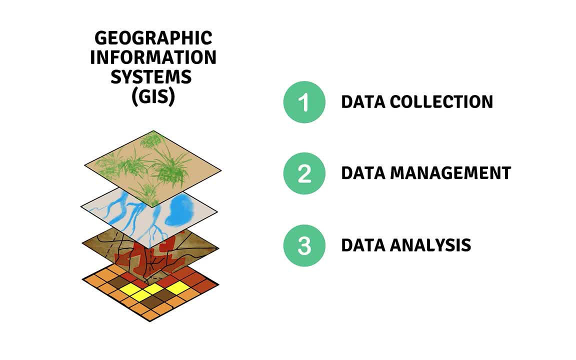 GIS can be referred to as a framework or a technology field or a computer system that is capable of collecting, managing and analyzing spatial data. I want to once again stress on these terms, which are collecting, managing and analyzing spatial data. Here, by spatial data, we mean information on the location. 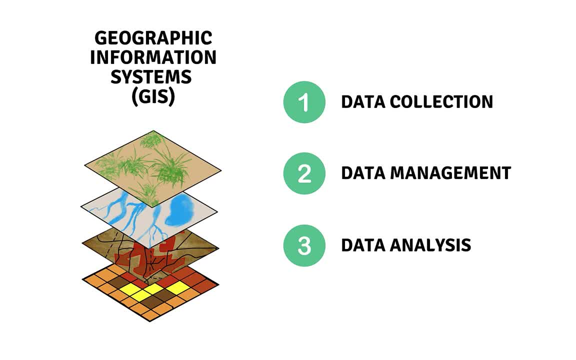 which is usually geographically geo-referenced, and all the information collected can be visualized as a map as well. So how is the data collection done? This can be using your phone or a GPS tracker, or using surveying tools, or maybe digitizing an old map that you already have. 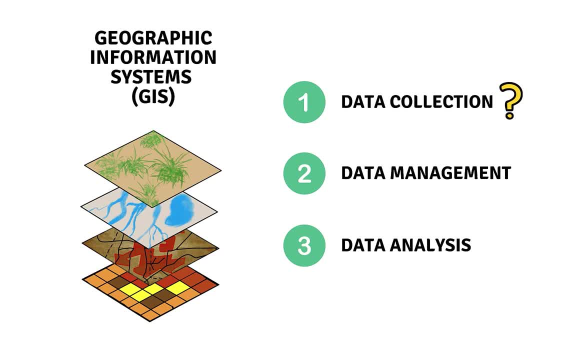 or just based on your knowledge of the area, you can add an information to GIS. All this data can be classified further into two main categories: vector and raster, which we'll be looking into towards the end of this video. We'll also be looking into various other key terms. 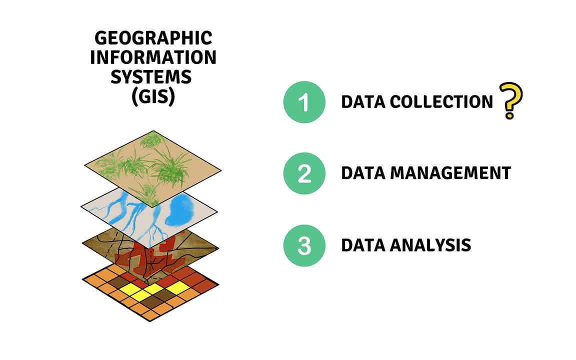 such as shapefile and geodatabase, because these are how the data collected is managed within the GIS. The data management part is also a very crucial element, as a lot of information coming in might be from diverse sources. For instance, there might be a part of your team out there. 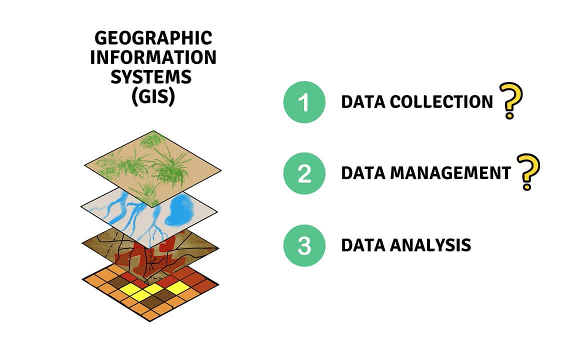 working in the field, collecting field data, and you'll be at the office working on the data collected in real time. For making this possible, GIS makes use of hardware and software capabilities, and you at times might need really powerful computers and servers to perform these operations. 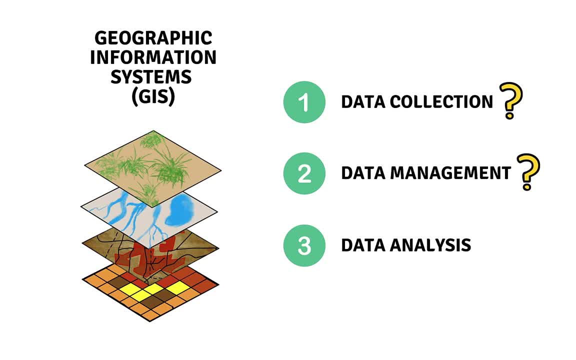 As you can imagine, apart from managing and storing the data, this step can also include enhancing the quality of collected data, as well as sharing the data to a wider audience. So once you have the data in a usable quality, then we can perform videos analysis. 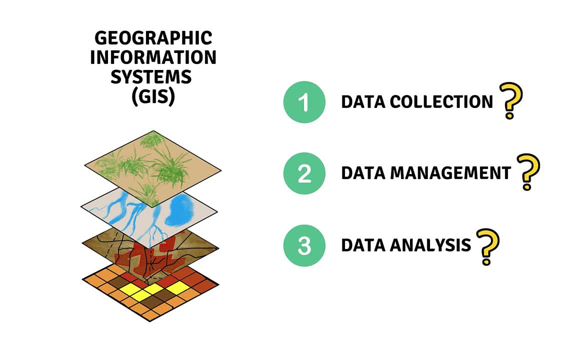 based on our research questions and then can further examine and refine results accordingly. If we take the example from before regarding buying a new house and if we want to know how far the nearest airport is, we can choose some analysis related to distance calculation in GIS. 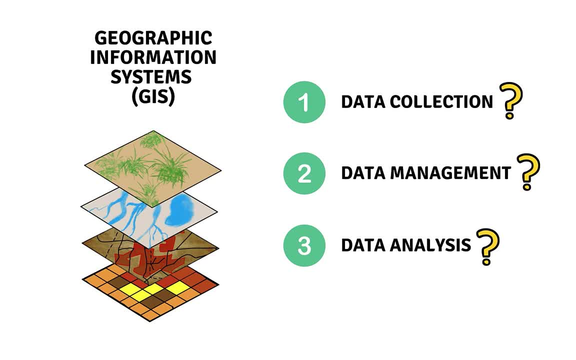 and easily come up with solutions And, based on the available traffic data, we can further optimize the route to reach the airport depending on the time of the day. This is exactly how Google Maps provide you with suggestions while driving during the rush hour time. 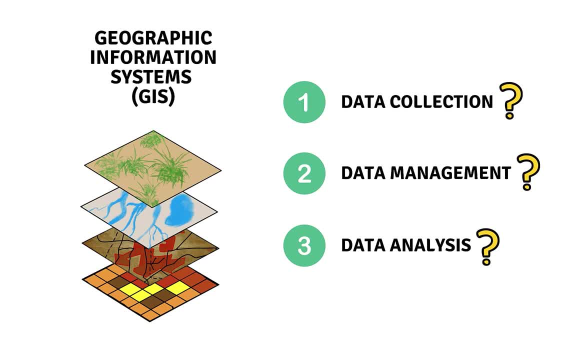 So, to summarize, GIS is a computer system that is capable of collecting, managing and analyzing spatial data, And few of the major components of GIS that you need to keep in mind are hardware, software, data, people and methods. Now that you have learned what GIS is, 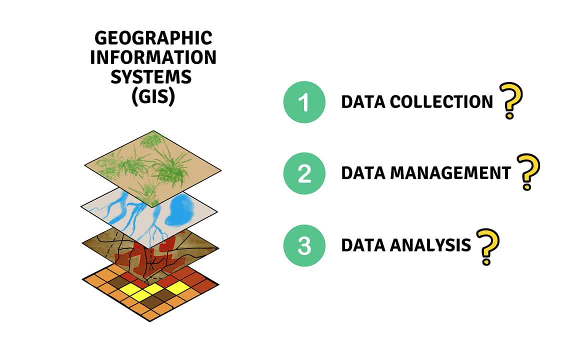 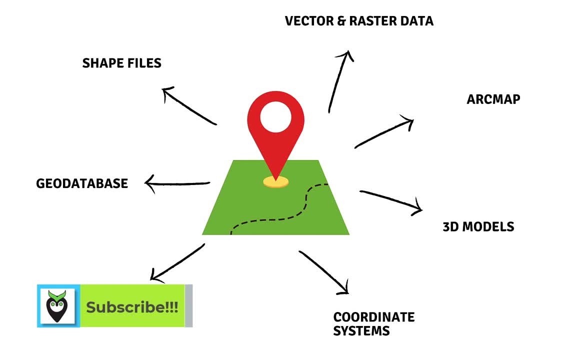 let's look into some key terms regarding this wheel of study before we wrap up this video. But before that, please make sure to smash that like button if you are finding value through this video. Okay, here I have come up with one, two, three, four, five, six, seven key terms. 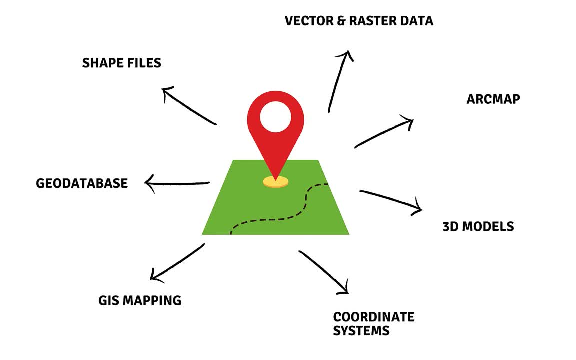 that you will come across again and again while stepping into the GIS arena. Let's start with vector and raster data, which are the two main types of data. Raster data can be treated as an array of grid cells, where each cell will be assigned a pixel value. 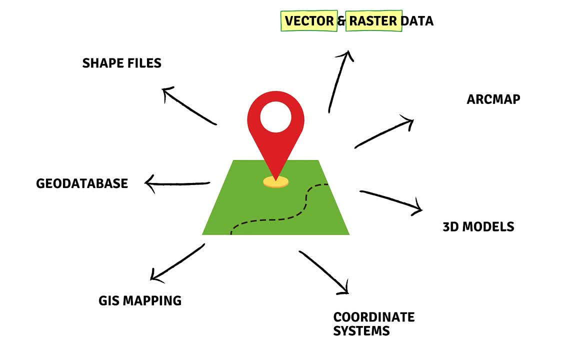 These can represent discrete entity types, Such as population density, or can be something like a continuous variable, such as temperature. The aerial and satellite imagery we bring into GIS platforms are automatically treated as raster objects, And this is one reason why, to me, 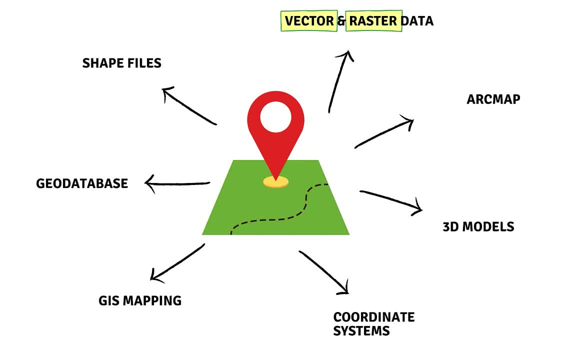 raster data is more associated with the remote sensing sector, And I usually link GIS with vector data analysis, because that's the real power of ArcGIS and those kind of platforms, at least from my understanding. While working with GIS, it is also very likely that you will be engaging. 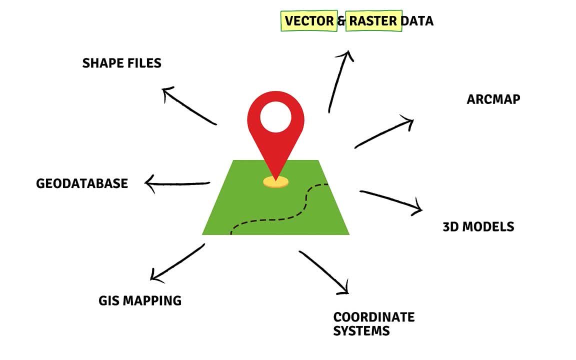 with vector data most of your time. So vector is a type of spatial data that uses x and y coordinates to define a location and can be further classified into three categories: points, lines and polygons. This brings us to our next term. 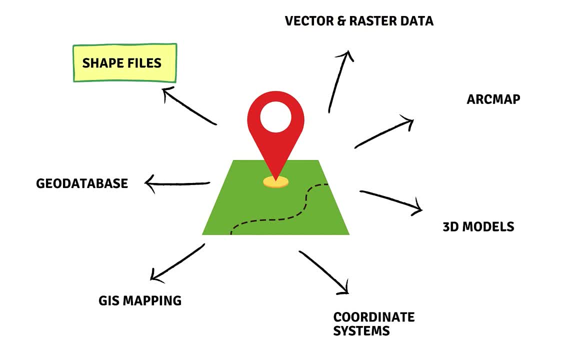 which is Sheffield. Sheffield is like the bread and butter of GIS. You will hear this every now and then. So what is Sheffield? Sheffield is a geospatial vector data format for GIS and is developed and regulated by ISRI, which is like the NASA and GIS sector. 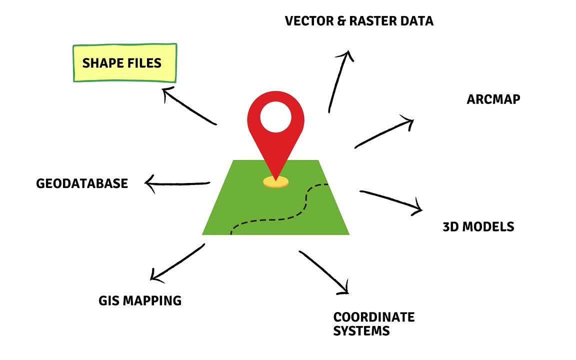 I'm sure that you would have heard about ISRI, since you are interested in GIS. They are a company based in Redlands, California, and is an international supplier of GIS software, Web GIS and all those kind of things- And ArcMap is the main component of ISRI's ArcGIS suite. 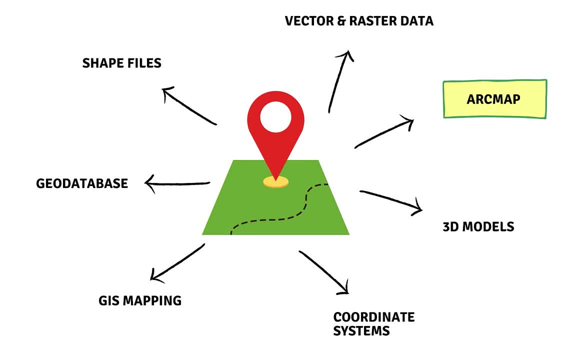 of geospatial processing programs and can be used to view, edit, create, explore and analyze geospatial data and more. Other than ArcMap, you can also find various other alternative open-source software. QGIS is one prominent example. 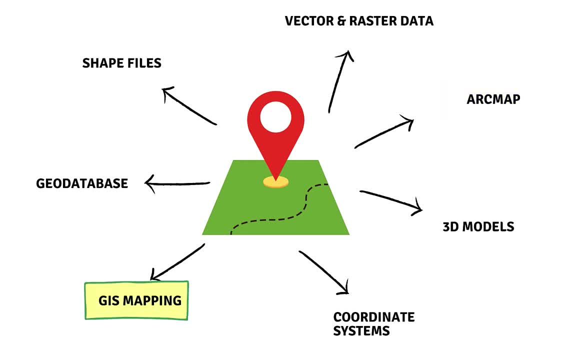 GIS mapping refers to the process of uploading data layers into a GIS software for producing specific maps that can provide valuable and easily readable information that raw data can present online, And while generating maps and performing spatial analysis, it is extremely important to keep a check on. 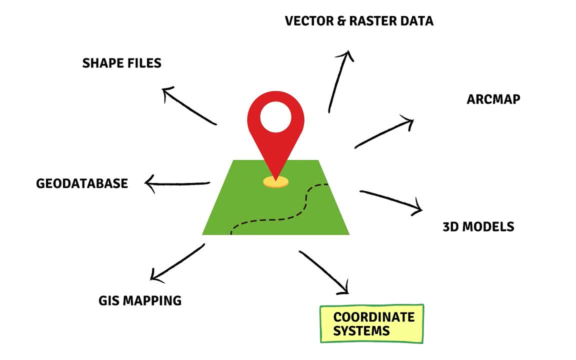 your projection coordinate systems, as otherwise the accuracy of your processes will be compromised. A geographic coordinate system is a way to define the locations on the surface of the Earth, and it uses three-dimensional spherical surface for this purpose. Within the GIS, this coordinate system information. 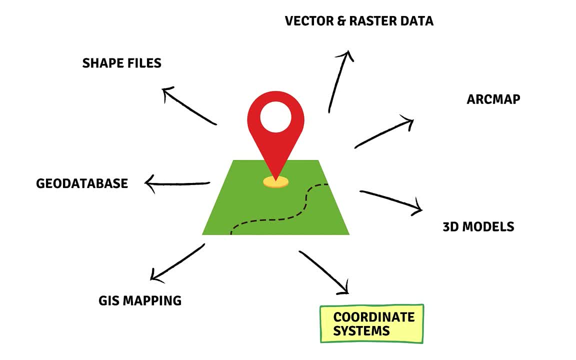 provides you with a framework of reference for your data and also helps with aligning your data with other existing data. Next is GeoDatabase, which we mentioned earlier. This is just a way to store large chunks of spatial data in a less messy manner. 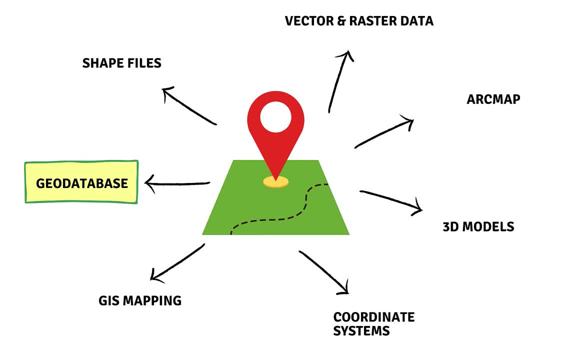 These databases are optimized for storing and querying data, and the information we put are hugely preserved and represented in the form of simple geometric objects such as points, lines or polygons. Finally, we have the 3D model, which can be generated based on the spatial information. 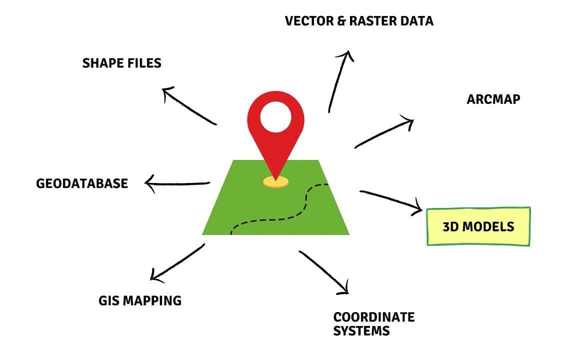 we had collected and processed within the GIS. This is a very interesting byproduct of GIS data and is extremely useful in sectors such as civil engineering and album planning. Nowadays, S3 even offers various interactive map options after creating 3D models to test different case scenarios.